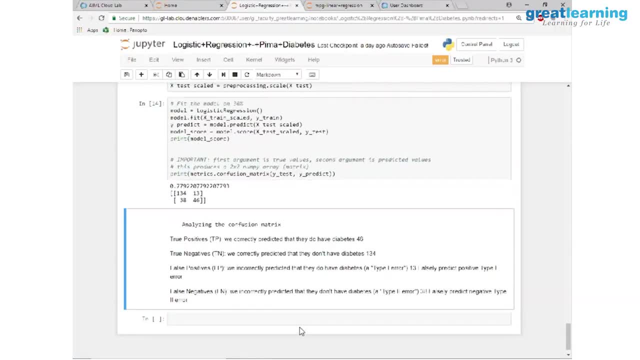 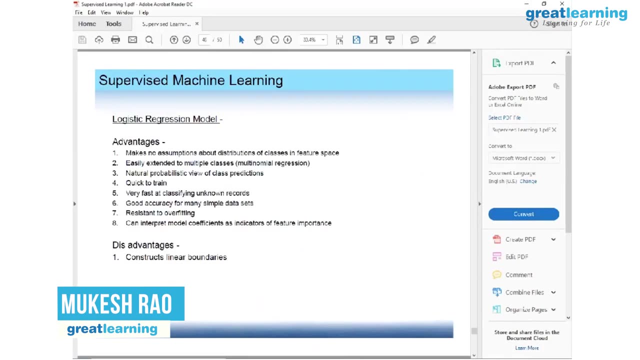 A brief introduction to logistic. Keep in mind logistic model is can be used for multi-class classification also. Now I have shown you only binary classification. here You will find these pros and cons about logistic. many other models Make no assumption about underlying distribution. 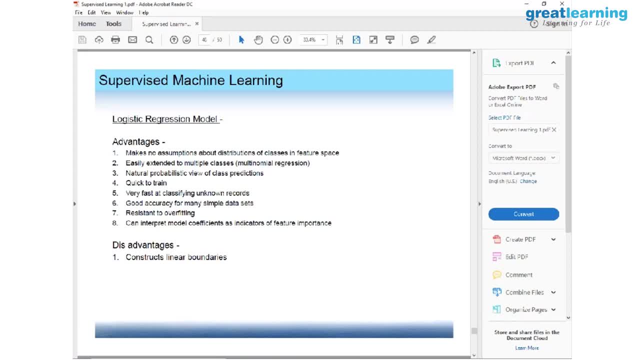 This is kind of you have to take with a pinch of salt. This is not really true in my opinion. Can be used for multi-class classifications. You can print out the probability values for each class. Given a query point, given an income: what is the probability? belongs to default or 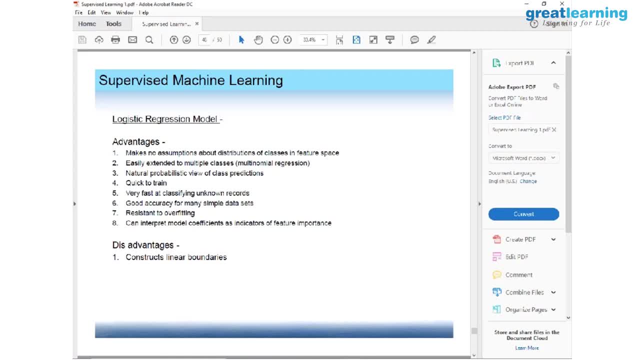 non-default. you can print out the probabilities also. Many people like that instead of class Relative to other algorithms. one of them which I am going to talk about, k nearest neighbors and all relative to other algorithms. this is quick to train And when the incoming record 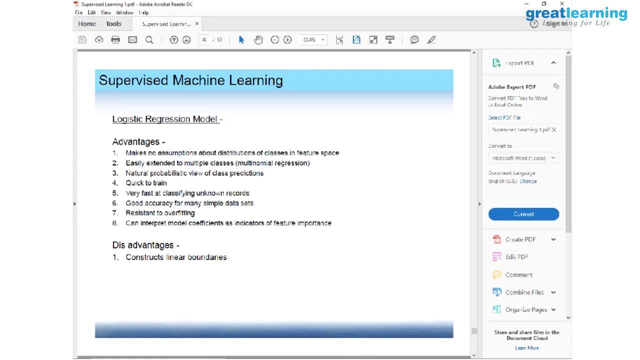 test record comes in, it is quick to classify. also, When you have simple data sets- simple data sets means dimensions which have clean classifications, Linearly segregating data points- then it gives you good results. But, as you saw, as long as you go with the default, resistant to overfitting, but then even this can be. 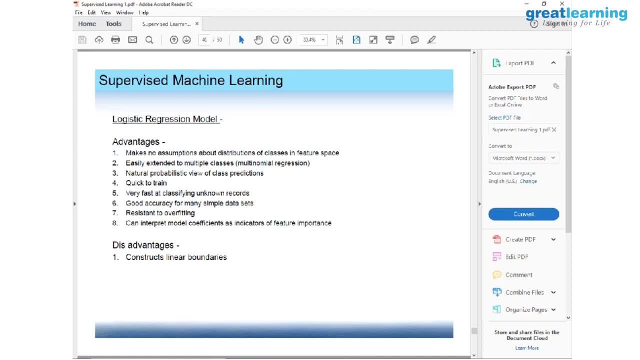 regularized. We can control this. also, All models can go to overfitting And, by the way, if you have any outliers, even this will fall on its face, Because inside this algorithm is linear model. Linear models are all impacted by outliers. If you print out the coefficients, 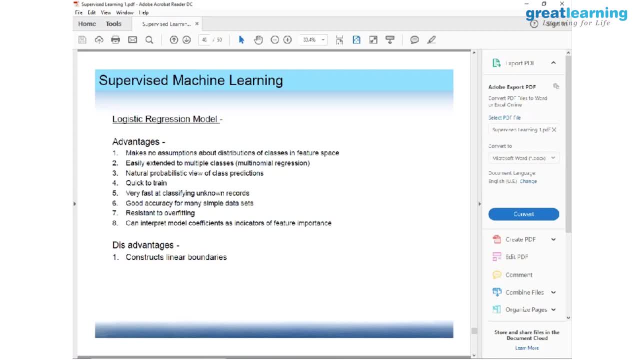 then you can make it. You will not be able to directly interpret this as we did in linear model. some people claim that this can be done. Disadvantage of this logistic model is again the way it cuts your mathematical space into boundaries, Since it uses underlying linear 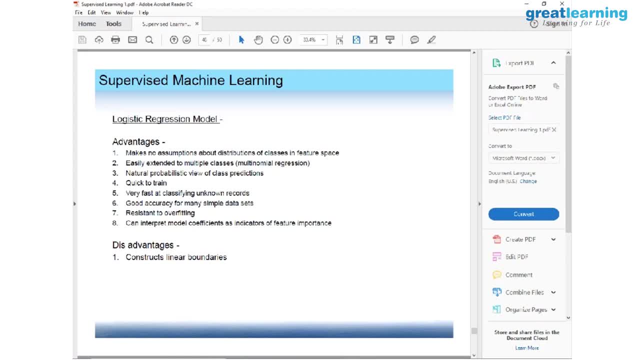 surface. that is a limitation. What exactly does that mean? We will see that when we do decision trees In multi-class classification also, this will be one versus the other. I have no problem. For example, Facebook's image recognition: the algorithm runs continuously. 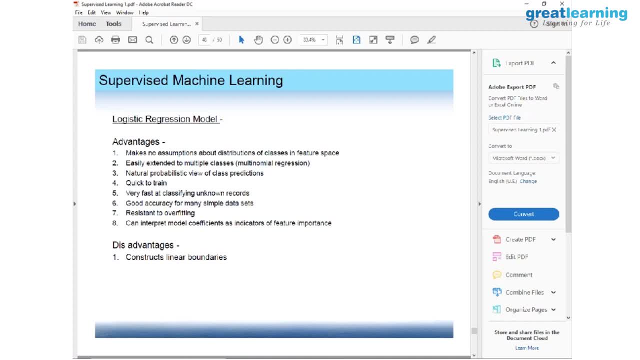 for six weeks non-stop before it learns to identify the images. But when it comes to quickly identifying on the fly a particular person, it takes no time. So training time or test time depends on that. So if it takes long time in training it is okay, But if it takes long,